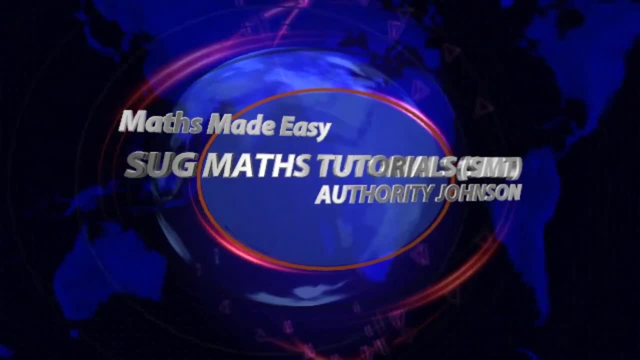 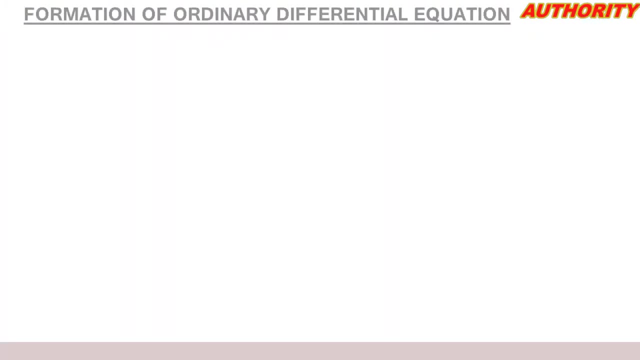 All right, you are welcome again Today. let's talk about formation of ordinary differential equation. Let's take a look at this question. We are asked to form a differential equation corresponding to this function. y is equal to a cos x plus 3, x plus 3 in bracket. Okay, 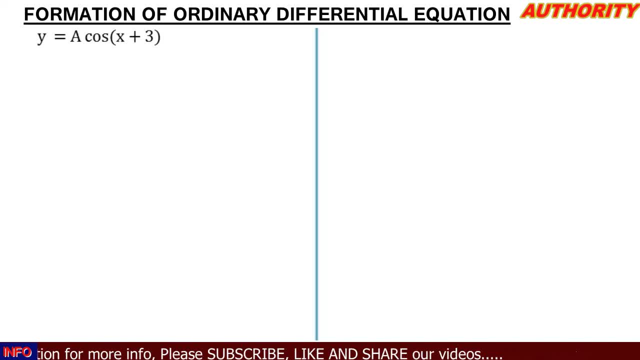 so we are asked to form a differential equation corresponding to this. Please pay attention, it's very simple Now. we have been emphasizing on the principle of formation of differential equation And we say that the principle holds good. That is the number of arbitrary constants. 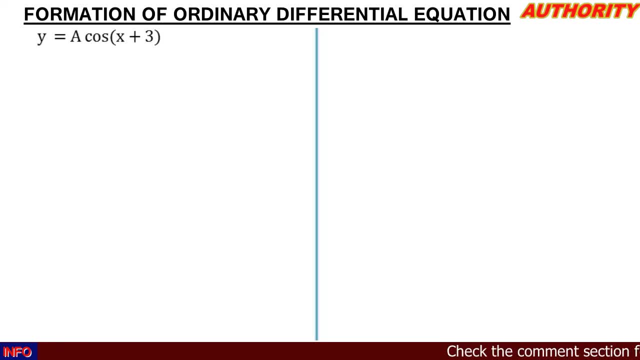 that is involved in a function determines the order of that differential equation. That is, how many arbitrary constants involved tells you how many times you are to differentiate that function in order to form the differential equation. If you have one arbitrary constant, that means you are to differentiate how many times 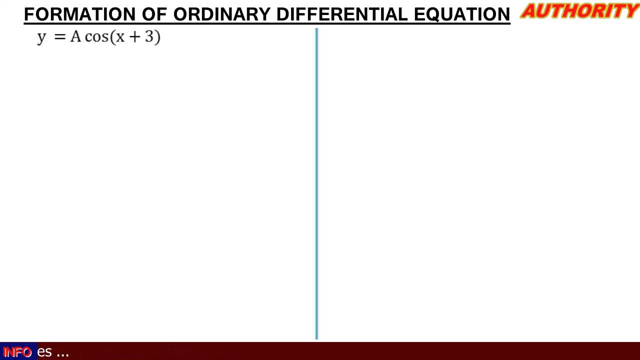 Once. If you have two, you differentiate two times, And if you don't have at all, you leave it that way. Okay, good, Now let's go Carefully. looking at this function we have now. y is equal to a cos x plus 3.. How many arbitrary constants do we have? We only have one arbitrary 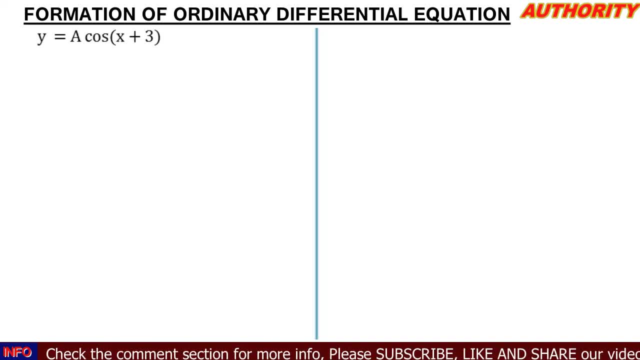 constant, which is what a. So we are going to try our possible best to remove this a. Okay, now let's go. The first thing we do is let's call this equation equation 1, and then let's differentiate. for the first, 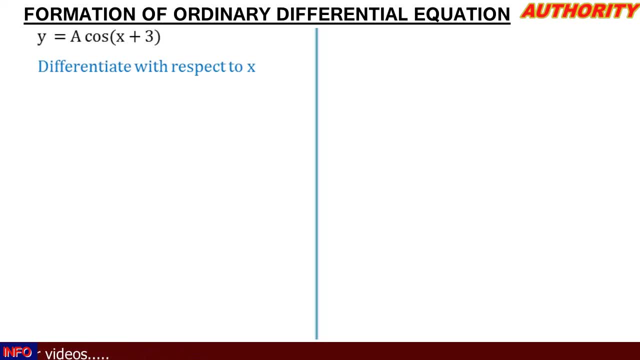 time When we differentiate for the first time, differentiating y with respect to x is going to give us dy. dx is equal to when we differentiate a cos x plus 3.. you know, a is a constant, okay, so differentiating this, what are we going to have? we're going to have 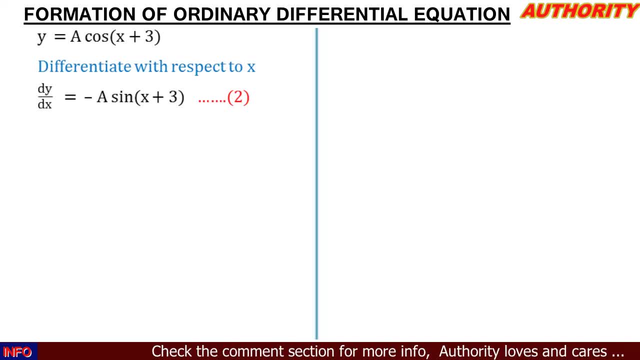 minus a sine x plus three. you get this right. so when we differentiate, cos x plus three is going to give us minus sine x plus three. so multiply by the constant which is a, so therefore we have minus a sine x plus three. you get this right. let's call this equation two. now let's go back to equation one. 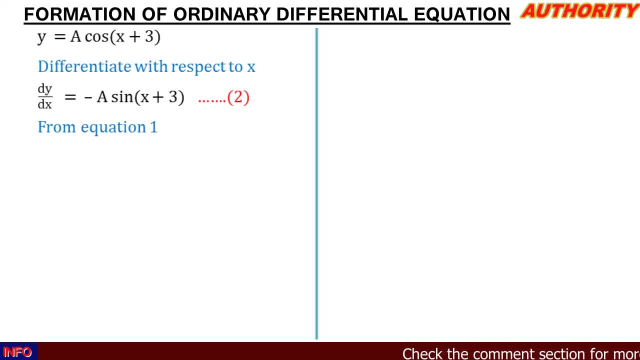 you know we are only to differentiate ones because we only have one arbitrary constant. okay, now going back to equation one. what do we have in equation one? we say that y is equal to a cos x plus three. in this place, can we make a the subject? yes, i think we can. now let's go, let's. 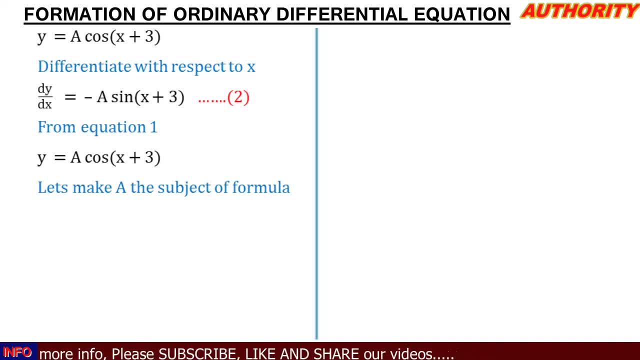 go ahead and make a the subject. so for us to make a the subject, that means we divide both sides by cos x plus three. then a will stand alone. so if we are to do so, we are going to have: y is equal to a cos x plus three, all over cos x plus three, and then the side of y, we say all over. 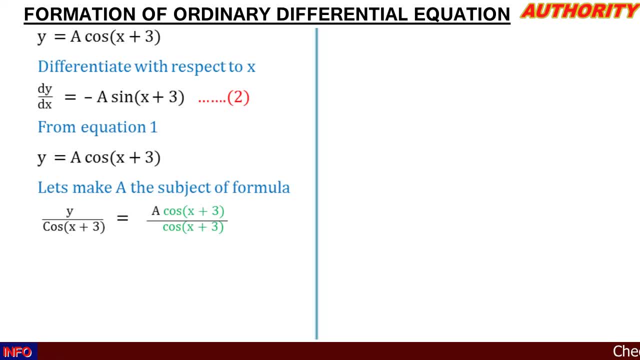 cos x plus three. okay. so in the side of a cos x plus three, we cancel cos x plus three. okay, so in the side of a cos x plus three, we cancel cos x plus three. so in the side of a cos x plus three, there will have a remaining in our right hand side, and then in our left hand side we have y all over. 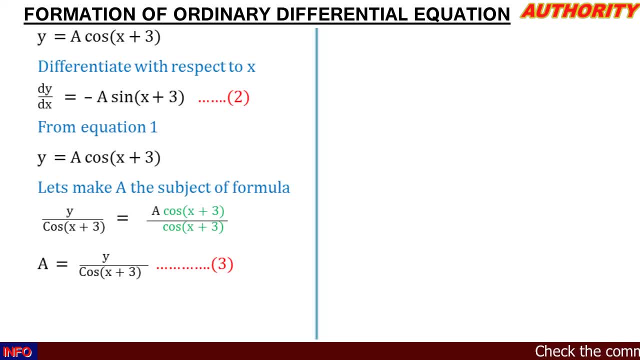 cos x plus three, permit us to call this equation three. okay, now we have equation one, equation two and equation three. carefully studying these three equations, we can see that we can substitute equation three into equation 2, because we used equation 1 to form this equation 3. okay, so we. 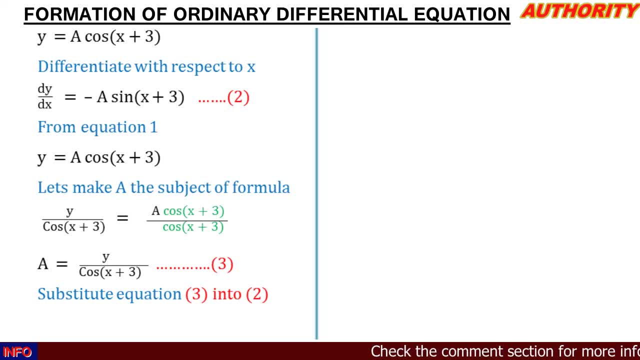 substitute it into the next equation, which is equation 2. all right, so what do we have in our equation 2? equation 2 says dy dx is equal to minus a sine x plus 3. now let's put minus by the side, put sine x plus 3 by the side, in place. 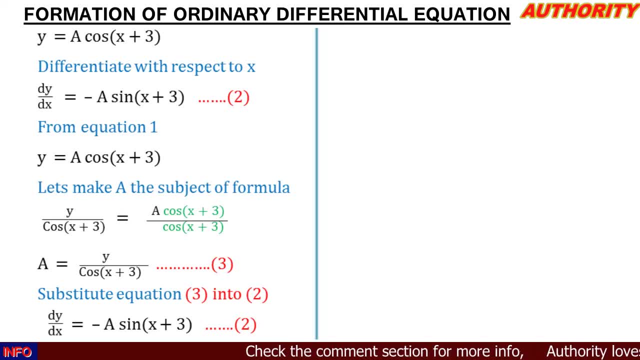 of a. we plug in the value y all over cos x plus 3. in doing so, we are going to have dy. dx is equal to minus double bracket y all over cos x plus 3. close the brackets: multiply by sine x plus 3. is it true? yes, now let's go. so if 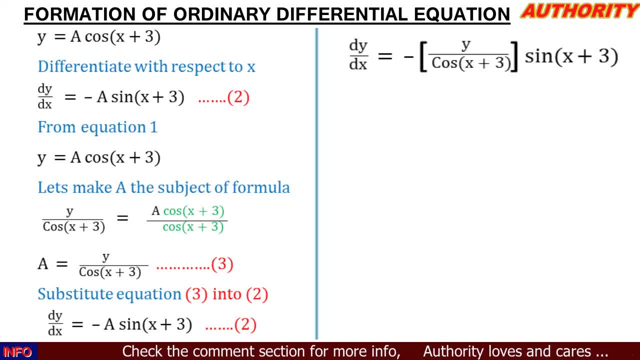 we open this bracket. or if you multiply everything now, we are going to have dy: the x is equal to minus y, y is equal to minus y. sign x plus 3 all over: cos X plus 3, is it true? yes, now let's like bring out. 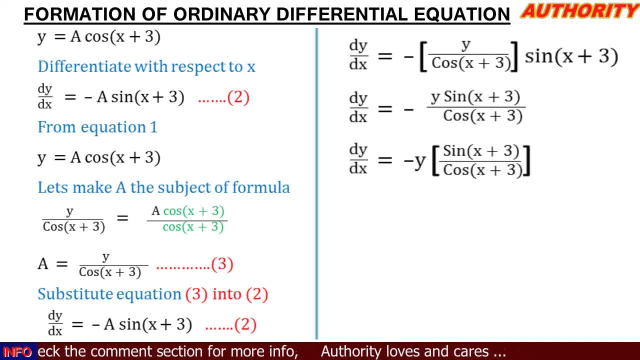 minus Y. now we're going to have dy. vx is equal to minus y in brackets sign X plus 3. all over cos X plus 3. you remember that sign all over cos is equal to what tan? so permit us to see: let tan X plus 3 be. 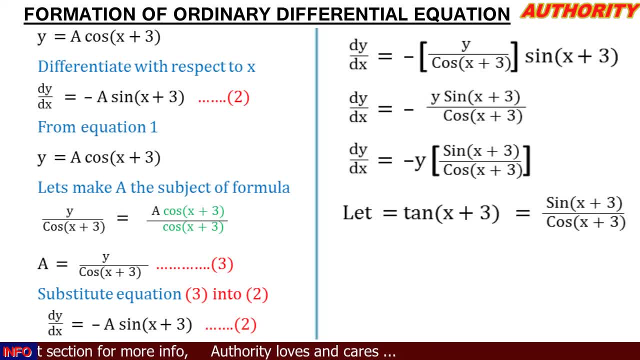 uine cos x plus 3. sin x plus 3 all over cos x plus 3 is equal to tan 3. cosine x be equal to sine x plus 3 all over cos x plus 3. so in the place of this, sine x plus 3 all. 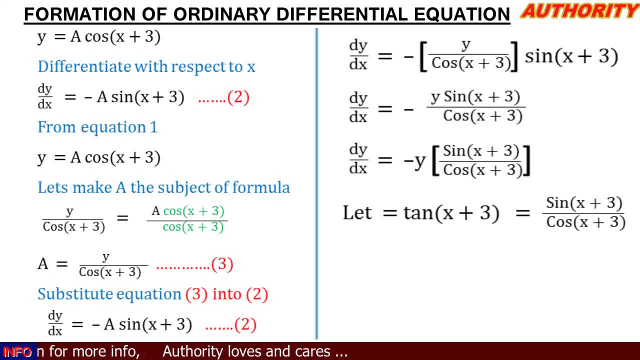 over cos x plus 3. let's replace it with what? tan x plus 3, because it's actually the same. okay? so if we do so, we are going to have dy dx is equal to minus y. tan x plus 3. we can rearrange by taking the terms to one side. so, doing so, we are going to have dy dx plus. 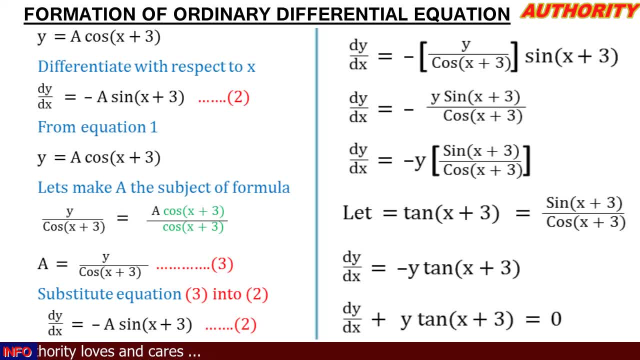 y, tan x plus 3 is equal to 0. hello, so here we say: dy dx plus y, tan x plus 3 is equal to 0. so therefore, this is the differential equation corresponding to the equation: y is equal to a cos x plus 3. all right, yes, thank you very much for watching, please, if you are. 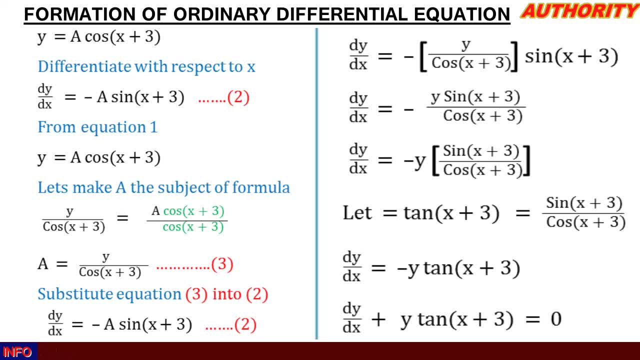 new to our youtube channel. this is svg math tutorial. please do well to subscribe, like the video and share. stay blessed, thank you.